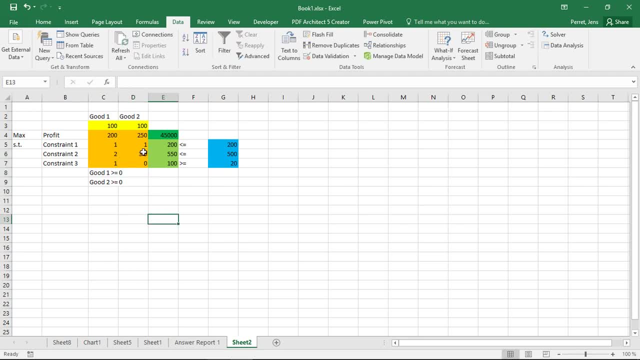 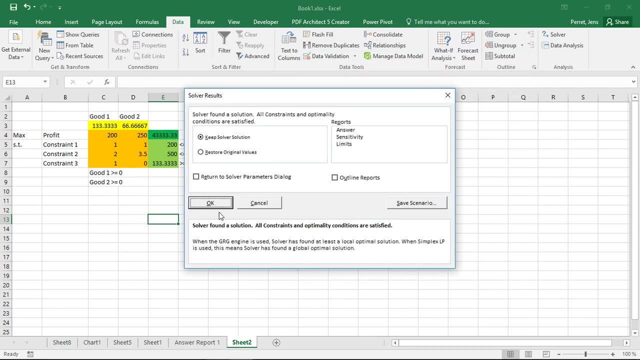 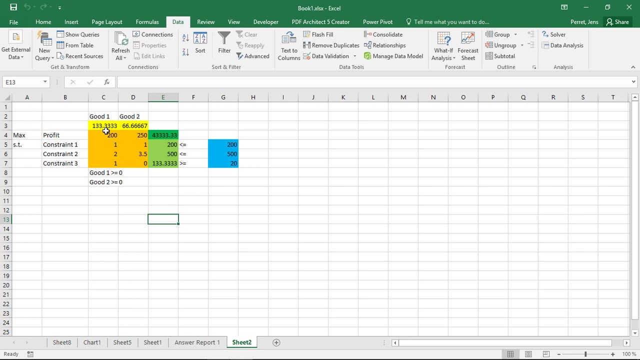 the requirements at this point. So now it takes not 3 but 3.5 units in context of constraint 2.. I solve this and now I see the problem. He tells me to produce 100, 33.33 units of good 1. Well, obviously this is not possible. The problem also is, if I just round, 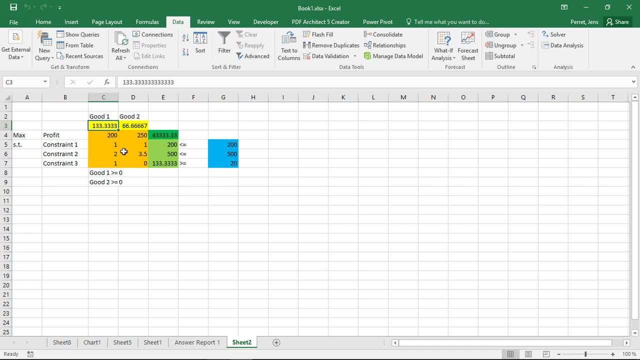 this down and this up. not necessarily does this have to work Here in this example. if I do it like this, I can directly see this point. I will not observe this constraint, So this will be a problem. just rounding this up and down. So what I have to do in this case is to round this up and down. So what I have to do in this case is to round this up and down. So what I have to do in this case is to round this up and down. So what I have to do. 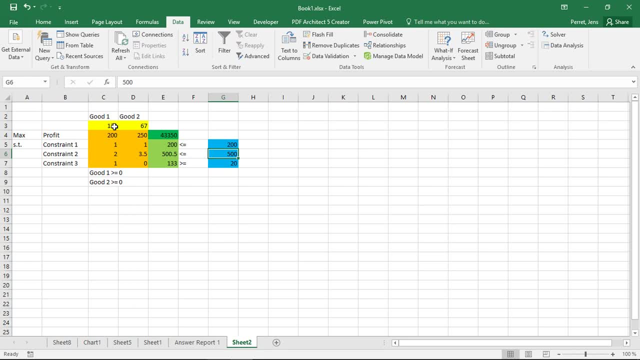 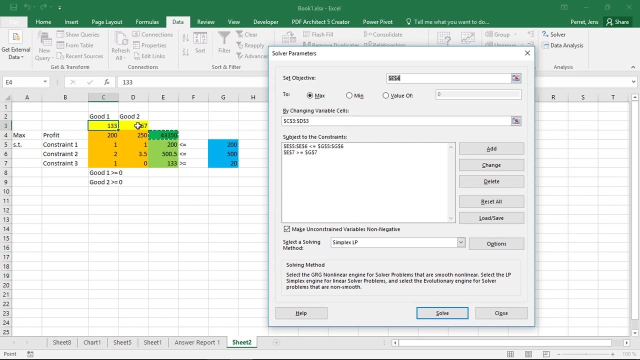 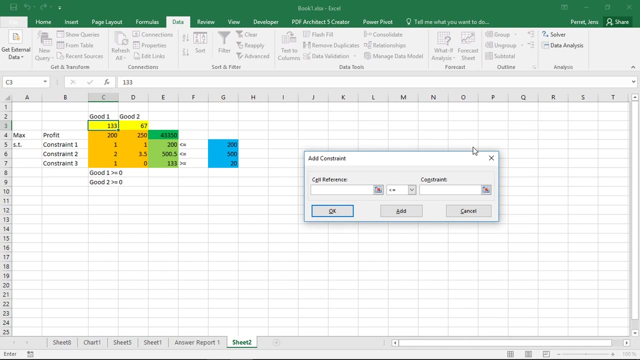 instead is actually solve this problem as an integer optimization problem, And this can easily be done. The advantage is here: I already have everything entered. So if I want to transform this real valued problem into an integer problem, I just go to constraints and I add one constraint. 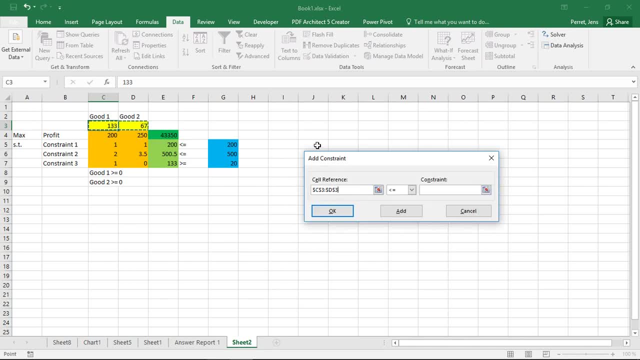 And that is on the left, I select all my decision variables, And that is on the left. I select all my decision variables And then in the middle where I select the type of constraints I'm going down here, And then I have two possibilities. The int actually means I have integers. 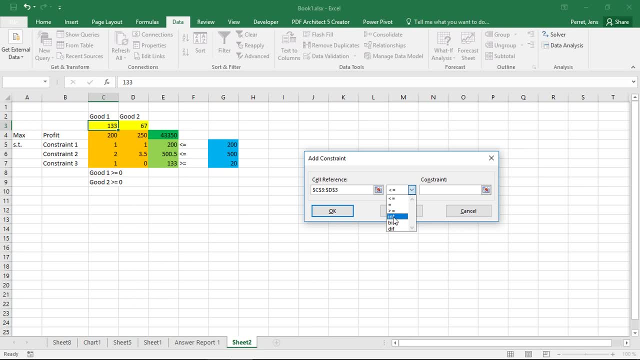 So whole number inputs, So 0,, 1,, 2,, 3,, 4,, 5, whatever. And the bin means I have binary inputs, So 0 or 1.. Well, here I actually want to have integer inputs. So that's basically all I have to do. 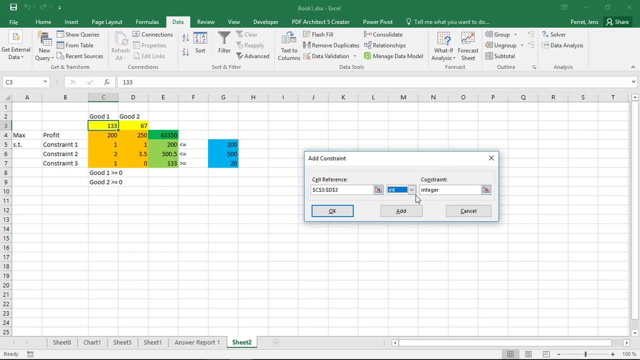 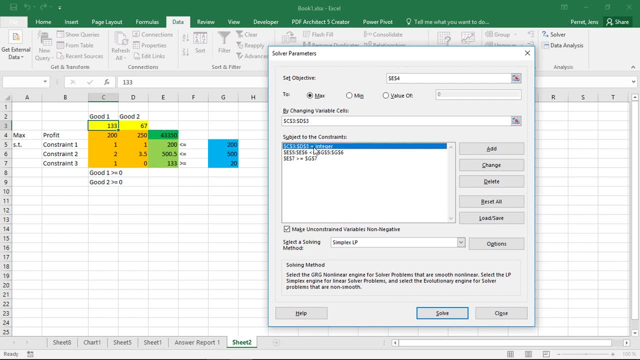 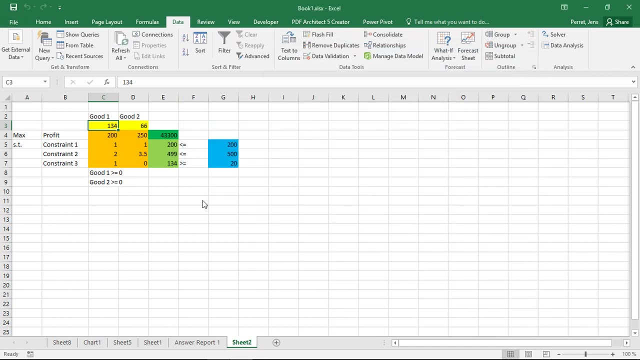 Select this. Then here he directly says they are to be integers. So I click OK And this condition is added as a constraint, so he will find a solution where both of them are integers, Click solve. You see, here that's my solution and as compared to what I did, he actually rounded the first one up and